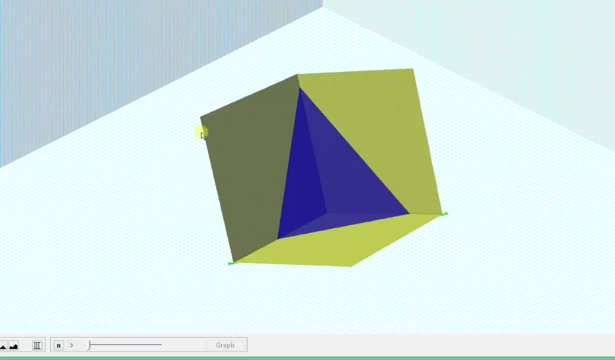 bounded by the blue plane and the three yellow planes, which are the three coordinate planes. So our goal here is to find the volume of this tetrahedron. Now, if we didn't have graphing software, we'd still want to graph this. 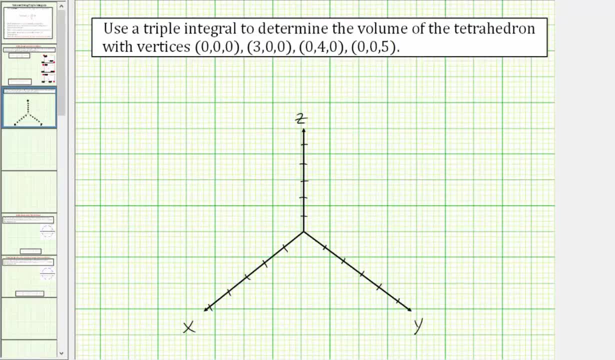 So, using the x, y and z axes, we would plot these four points. So we have this point here at the origin. The x-intercept is three comma zero, comma zero here. The y-intercept is zero comma four, comma zero here. And the z-intercept is zero, comma zero, comma five, which would be here: 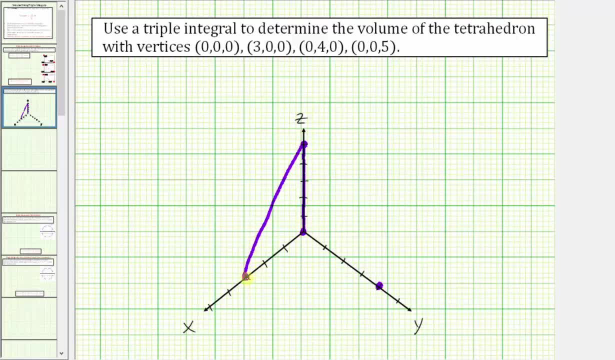 So this would be the tetrahedron, Again that we're trying to find the volume of Notice, how it's bounded by the first octant, or the three coordinate planes, and this plane here where we know the three intercepts. 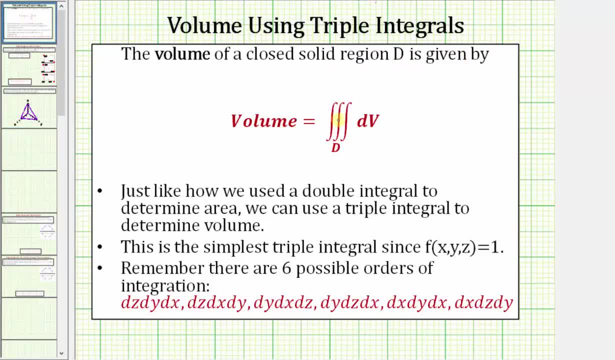 The volume of a solid region D is given by this triple integral, where we integrate over the region D, which again is the closed solid region. Notice how the integrand function is just one and differential v can be any of these six possible orders of integration. 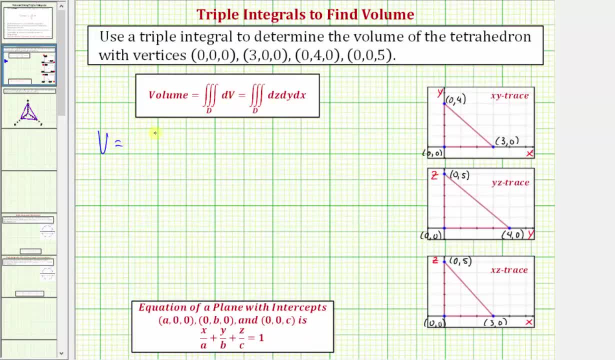 So let's go ahead and set this up as the volume v equals the triple integral, And let's go ahead and include one as the integrand function. And let's use the order of integration, of integrating with respect to z first, then y and then x. 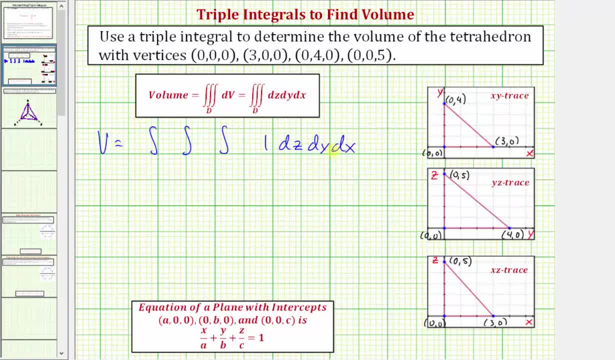 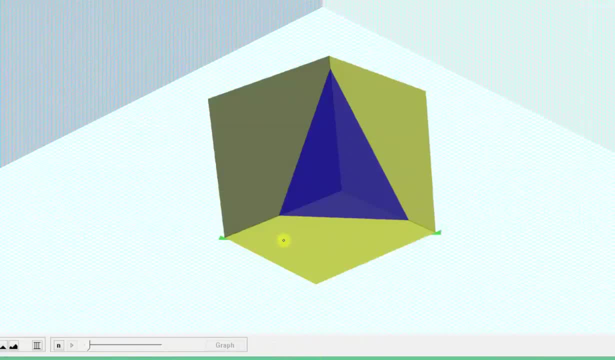 Any order would work, but let's go ahead and use this order of integration. So now we'll determine the limits of integration for z. We'll notice how the solid is bounded by the xy-plane, which would be: z equals zero, and it's bounded above by this blue plane. 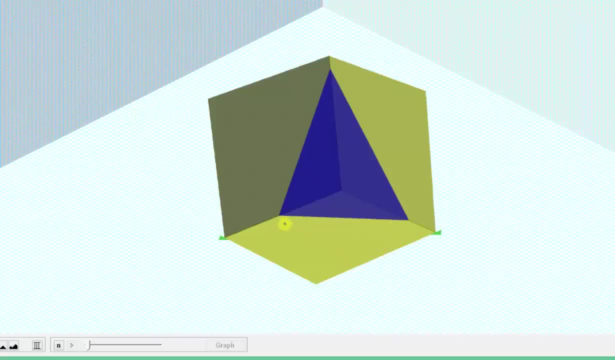 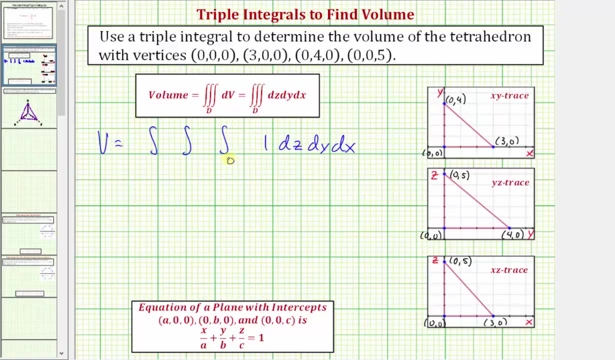 So now we need to find the equation of this blue plane, which we can do because we know the equation of the intercepts. But again we know the lower limit of integration with respect to z is going to be zero And the equation of the plane with these three intercepts is given by this equation. 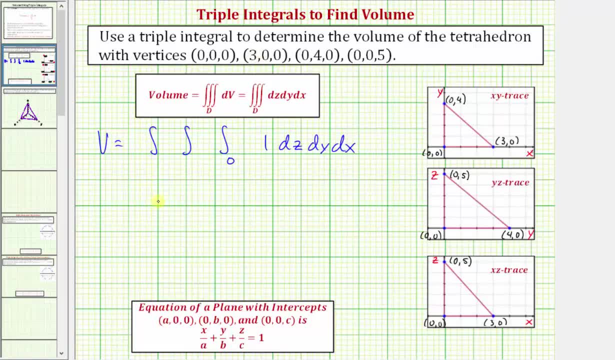 So because the x-intercept is three, we're going to have x divided by three plus the y-intercept is four. so we have y divided by four plus the z-intercept is five. so we have z divided by five equals one. 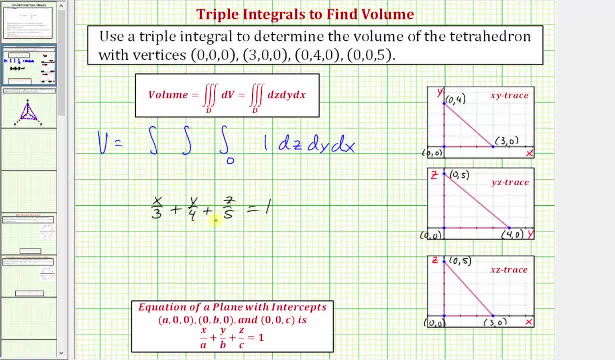 And now, if we solve this equation for z, we can determine the upper limit of integration for z. Now, if we integrate with respect to a different variable first, we'd have to solve this equation for whichever variable we integrate with respect to first. But we'll solve this for z, so we'd have 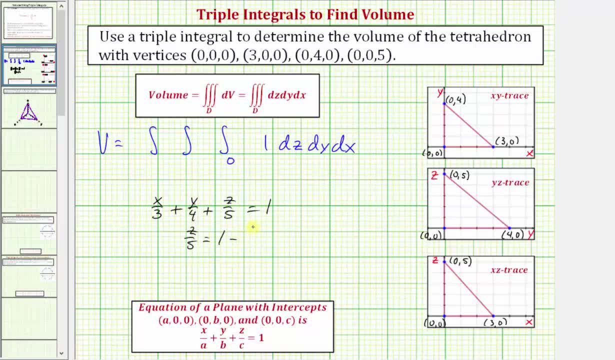 z divided by five equals one minus x divided by three minus y divided by four. And now I'll multiply through by five, so we have z equals five minus five-thirds x minus five-fourths y. Again, this is going to be the upper limit of integration with respect to z. 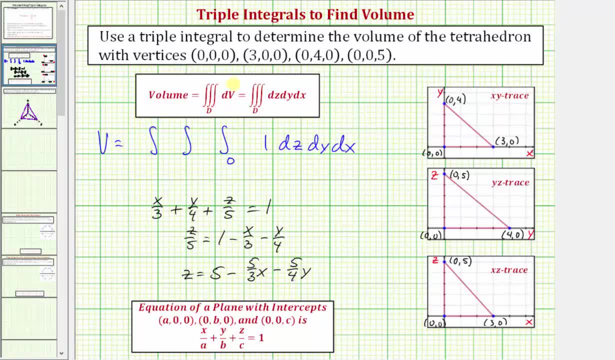 And notice how we have z expressed in terms of x and y. So we have five minus five-thirds x minus five-fourths y, And now we need to find the limits of integration for y and x. To do this we'll want to have the x-y trace In general to determine the x-y trace. 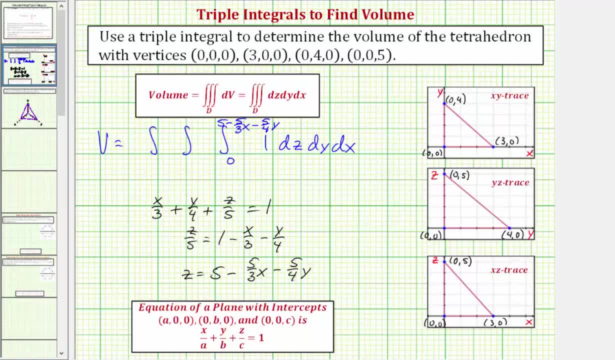 we set z equal to zero. So notice, if z is equal to zero for these four points, we'd only have three points to consider: zero-zero, three-zero and zero-four. And I've already plotted these three points in the x-y plane so we can determine the limits of integration for y and x. 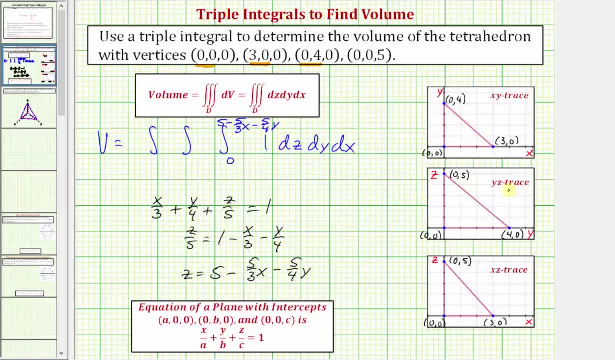 using this triangular region. here I also included the y-z and x-z traces. We don't need those for this example because of the order of integration that we're using, But if we change the order of integration, depending on the order, we'd have to use one of these traces instead. 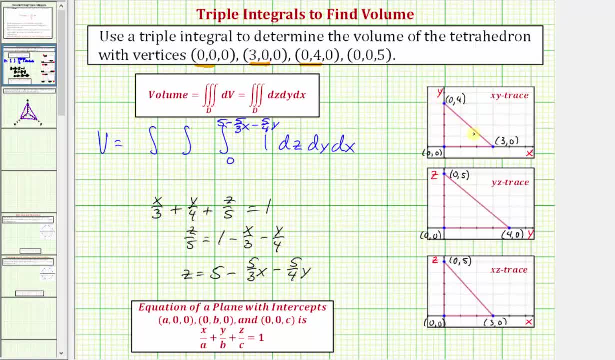 We're going to need the equation of the line that contains this side of the triangle. There's two ways of doing this. We could set z equal to zero and solve this equation for a y, which would take some work. It's much easier to recognize that the vertical intercept is four. 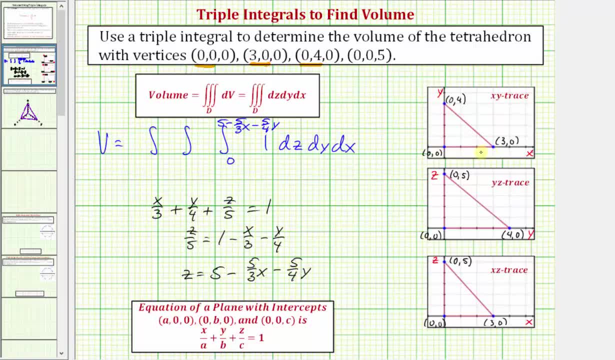 and the slope would be down four right three. So the slope is negative four-thirds. So the equation of the line containing this side of the triangular region would be: y equals four, the vertical intercept minus four-thirds x. So with respect to y, we integrate from y equals zero. 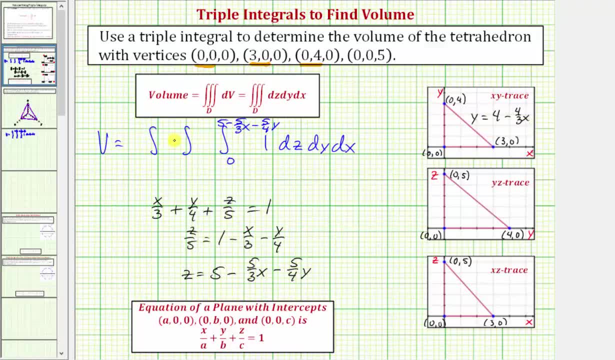 to y equals four minus four-thirds x. So again we have from zero to four minus four-thirds x. Notice how we express y in terms of x. And again these are the limits of integration. for y, because this area in the x-y plane is bounded below by y, equals zero. 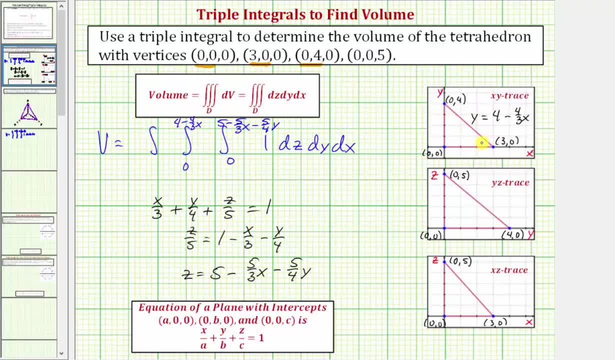 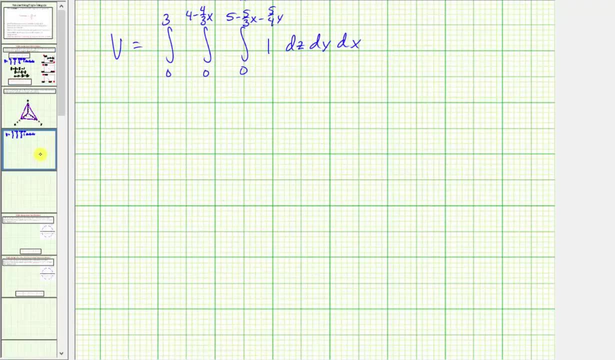 and bounded above by y, equals four minus four-thirds x. And finally, the limits of integration for x would be from x equals zero to x equals three. So this triple integral will give us the volume of the tetrahedron. Let's evaluate this on the next slide. 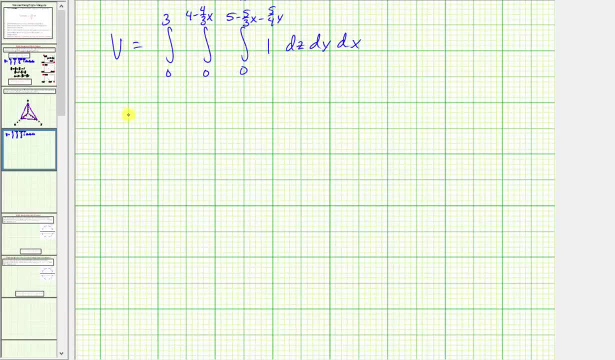 So we first integrate one with respect to z, which would just be z. So we have the double integral and again the antiderivative is z. Notice, when we evaluate big F of b minus big F of a, we're just going to have this quantity. 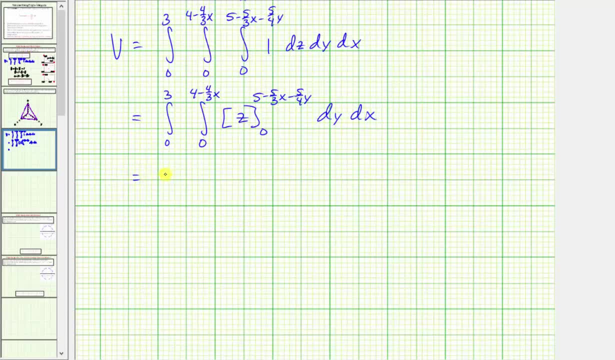 minus zero, which means for the double integral, the integral function is just going to be the quantity five minus five-thirds x minus five-fourths y. Now we integrate with respect to y, treating x as a constant. So we'd have five y minus five-thirds xy. 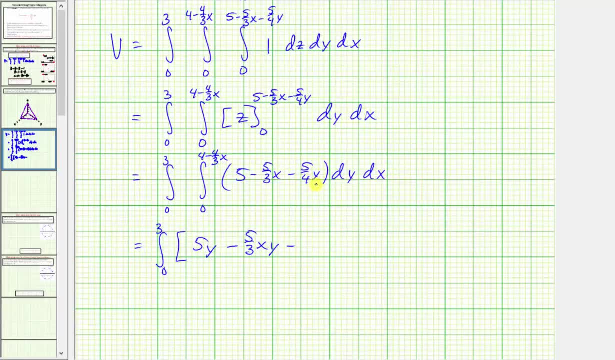 and then we'll have minus five-fourths times y-squared. divided by two or five-fourths times one-half y-squared, That'd be five-eighths y-squared. Now this starts to get messy. We need to find big F of b minus big F of a. 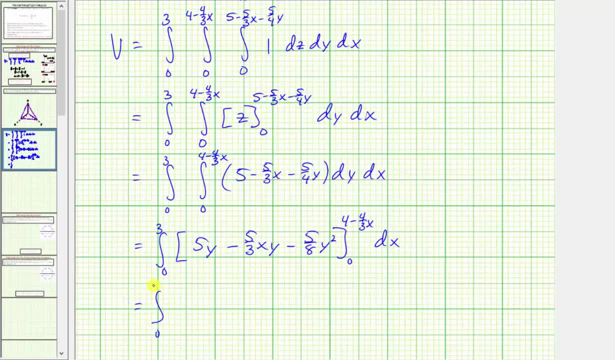 So we'd have the integral from zero to three of. we substitute four minus four-thirds x for y, so we'd have five times the quantity four minus four-thirds x, minus five-thirds x, times four minus four-thirds x, and then minus five-eighths. 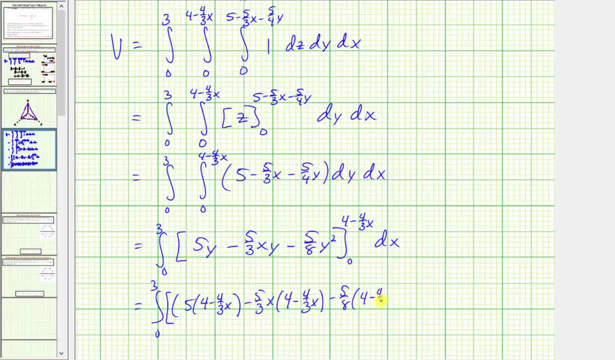 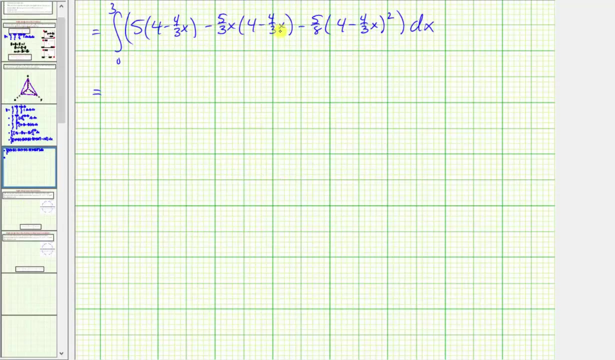 Times the quantity four minus four-thirds x-squared, There's big F of b, and then for big F of a, of course each of these has a factor of y, so we'll just get zero. Now let's go ahead and simplify all of this.